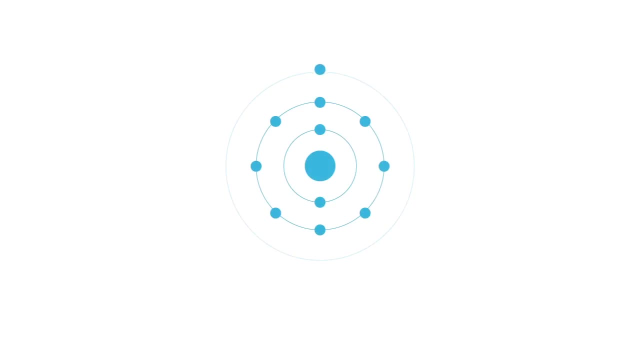 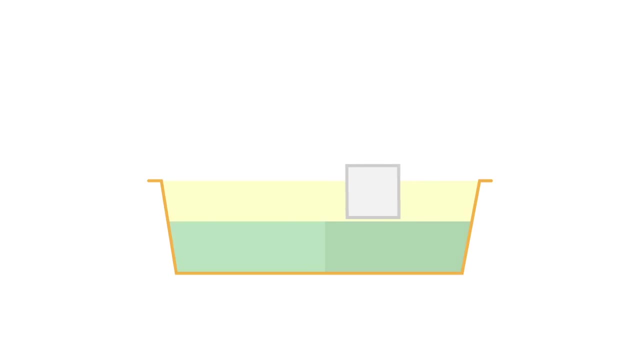 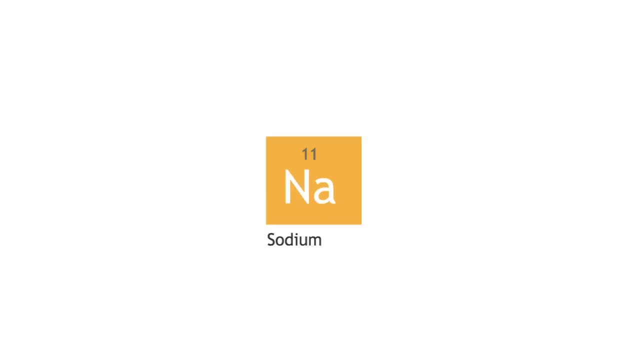 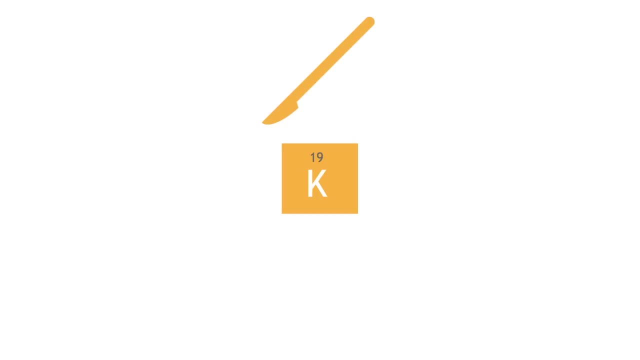 what predictions can you make about its softness and the vigor of its reaction with water in comparison with sodium? please pause the lesson to think about this and resume when you are done. you will find that potassium is softer than sodium and easier to cut. it reacts more vigorously with water than sodium. however, an important observation is made: it burns with a lilac flame. 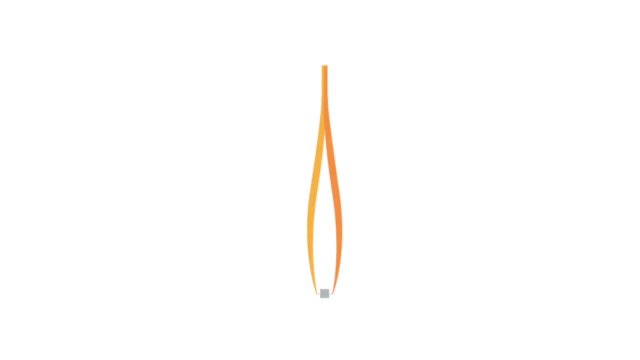 ure that a very small piece of joatacium is used and stand far back as it may spit. you may olso hear a small popping noise due to the os. lovely tal gaat fondso yov the resiton of hydrogen legen. All alkali metals float on top of water. 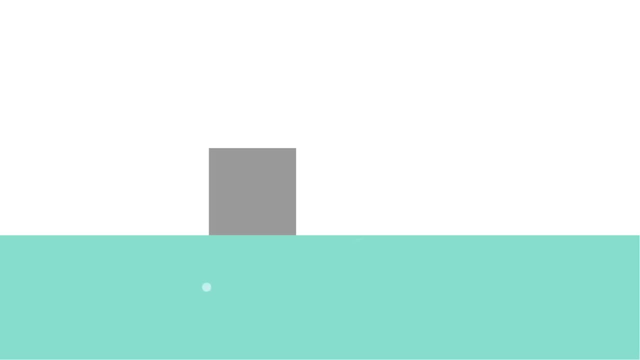 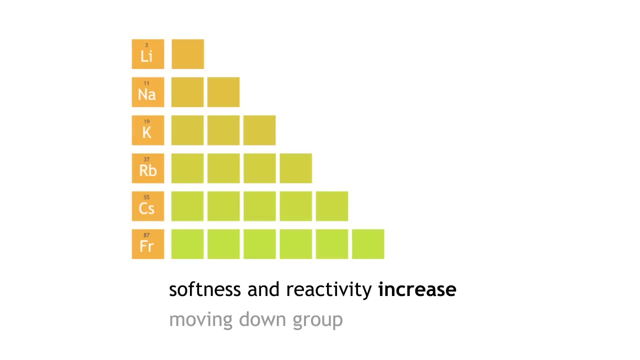 This is in contrast to the alkaline earth metals or the group II metals, which sink when they react with water. So, moving down the group, alkali metals become increasingly soft and react with increasing vigor with water. We can predict that rubidium and cesium will be much softer and much more reactive. 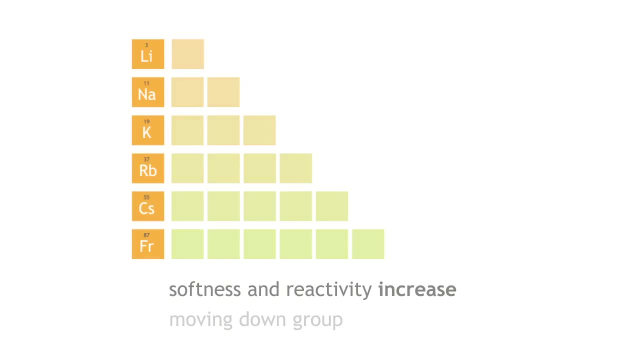 Strontium is radioactive and is very rare in nature. There are also other observed trends moving down the group. Their density increases and their melting points and their boiling points will decrease. In summary, the alkali metals are the group I metals. They react with water to produce hydrogen gas and their corresponding metal hydroxide. 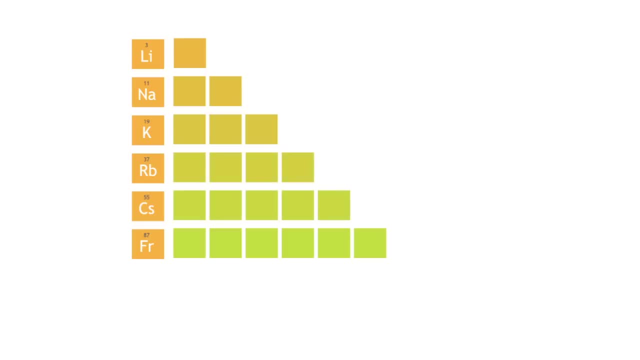 Moving down the group. softness of the metal increases, Reactivity with water increases, Their density increases, but melting points and their boiling points will decrease.